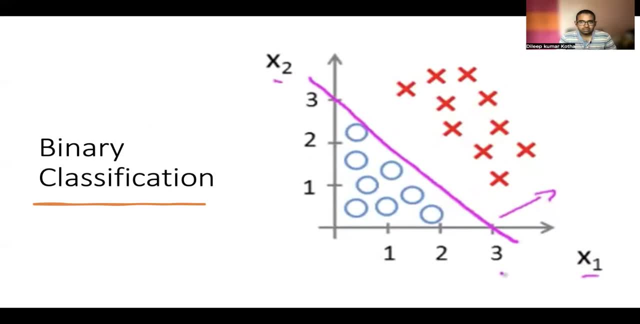 our hypothesis. That's all we need to determine a hypothesis where it fits- And this is decision wonder, which we discussed in the last video. And what is the hypothesis indicates in the binary classification? is it is a probability that, given a variable X, once you determine the 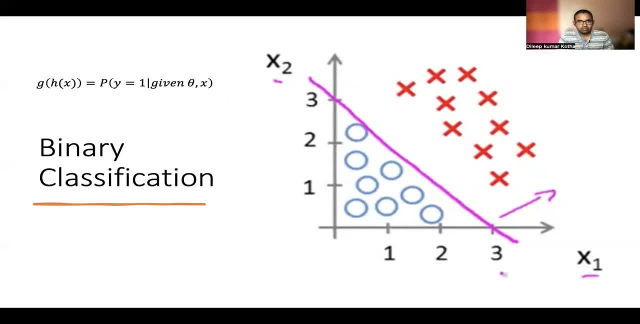 hypothesis using theta, whether it fits, belongs to a particular class. say, it belongs to class one, and if you want the probability that belongs to other class, you just need to subtract one minus from it. okay, so this is a sigmoid notation i have shown here. 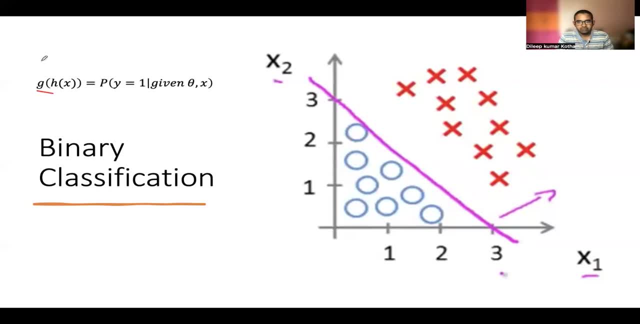 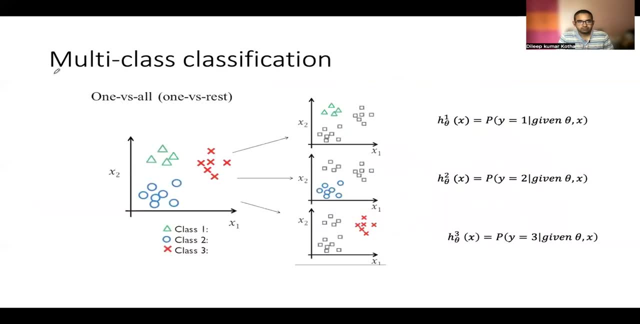 using the g, but normally the sigmoid notation and the hypothesis are used interchangeably once we move to logistic regression. now let's talk about multi-class classification. so here, instead of two classes, you have three classes. one is a triangle class, other one is a cross mark class, other one is a circle class. so let's call them class one, class two and class three. 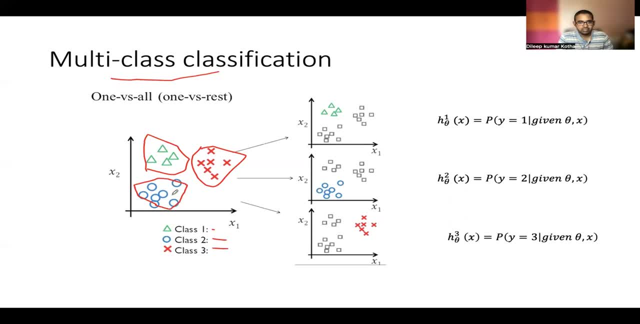 now what you do? whatever the class two and class three, you make them similar, so we take them to be squares. whatever class two and class three. now you can see this has converted into a binary classification problem. now we derive the hypothesis which will give us the probability that that 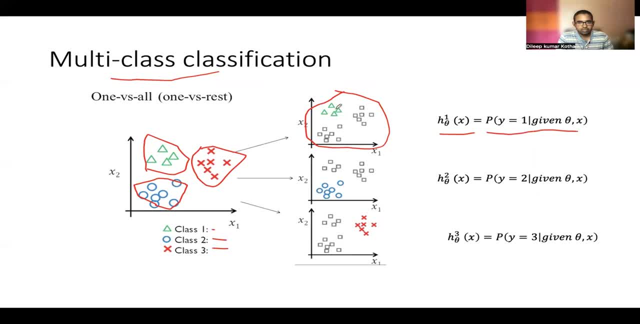 a given variable, x, when we predict it belongs to a triangle class. similar way in the second hypothesis calculation. what you do is you convert this triangular cross marks to another class. so now it is again a binary classification problem. now this second hypothesis gives us the probability that, given x, it belongs to the circle class. similar way for the third hypothesis.